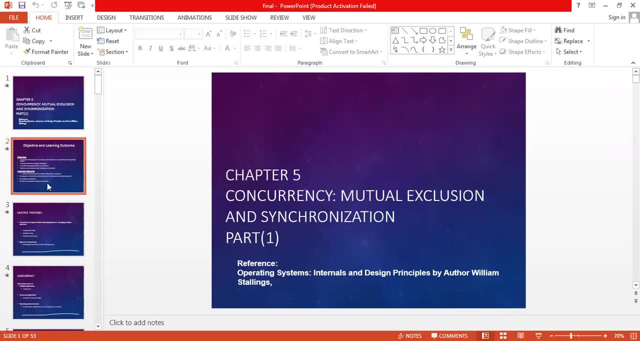 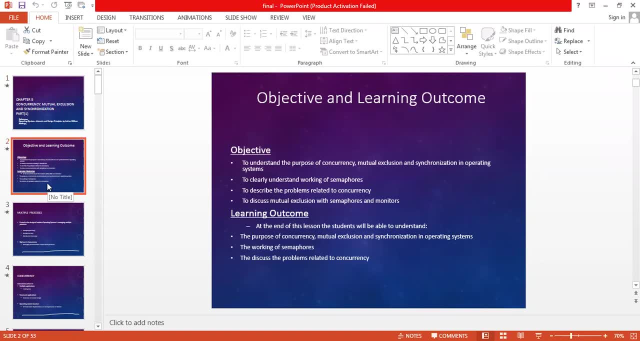 Objective and learning outcomes about my topic is to understand the purpose of concurrency- mutual exclusion synchronization operating system. clearly understand working of semaphores describing the problem related to concurrency. discuss mutual exclusion with semaphores and monitors. After completing my topic, you all are eligible to understand the concept of concurrency, mutual exclusion synchronization operating system, working of semaphores. 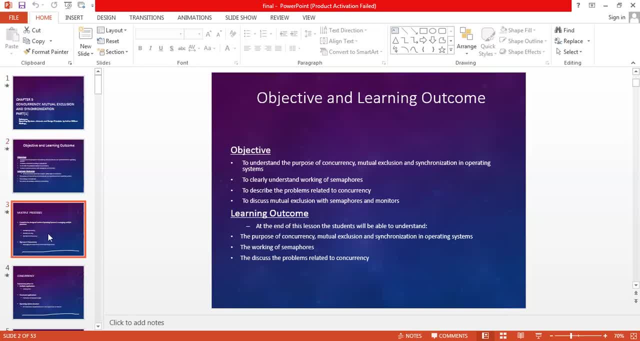 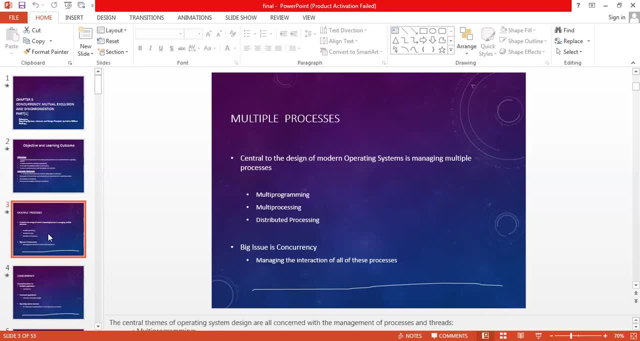 First topic is multiple process. Central to the design of modern operating system is managing multiple process: multi-programming, multi-processing, distributing processing. Big issue is concurrency, managing the interaction of all these process. When we are designing our operating system, we manage it so that we can run multiple process, multiple program, at the same time. 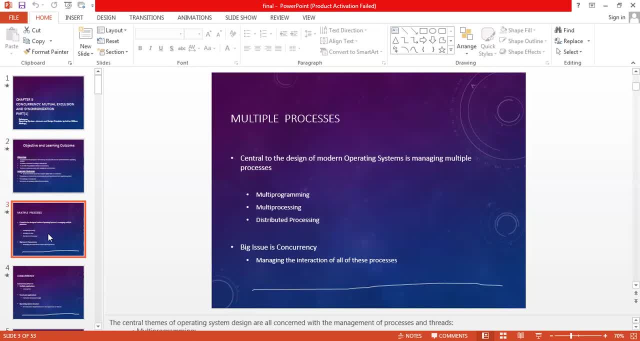 After multiple programming we can run multiple program In multiple programming. there is only one unit processor in which we are running multiple program In multiple process. there are more than one processor in which we are running multiple program In distributed processing. there are different processes, different processes, different processors, which we connect with each other, and then execution program is being done on it. 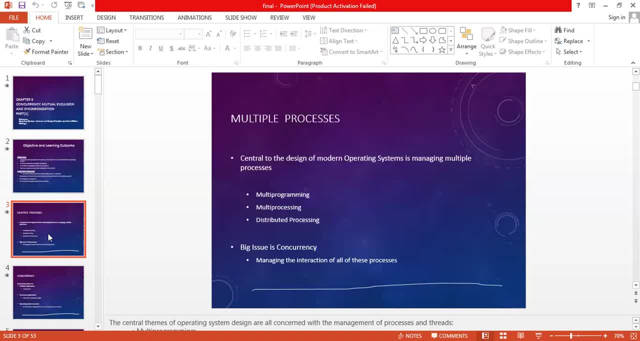 The main issue. there is concurrency in terms of managing multiple process. Which process is in execution state, Which process is blocked, Which process is in waiting, Which process needs which resources? In all these things we face the issue of concurrency. What is concurrency? 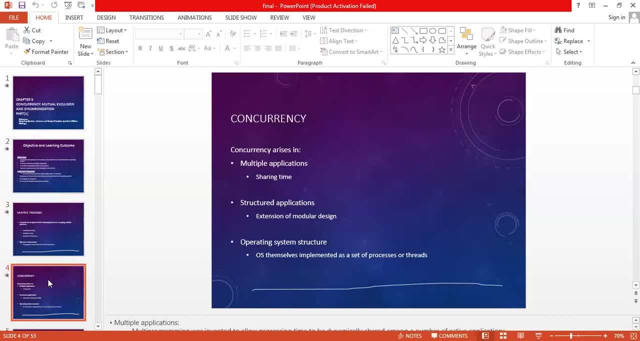 Concurrency arises from multiple application sharing. Structured application extension or modular design. operating system or OS themselves are implemented as set of processes or threads. Let's talk about concurrency. When we are using our system, computer, we open multiple tabs on the screen of our computer, on the screen of the system at the same time. 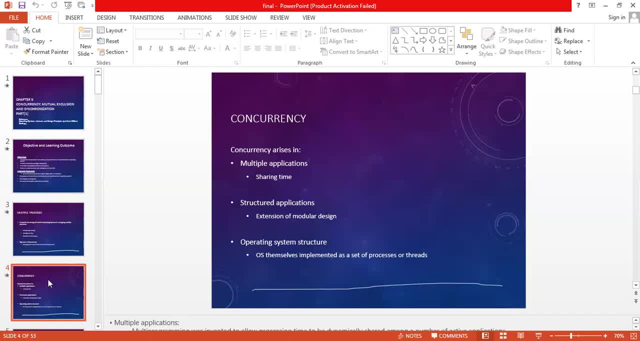 There is sharing of time. Structured application is an extension of modular design, That is, there is a separate module for each purpose, for each work, Which will perform only that specific work. After that, operating system structure. Operating system means that our OS is implemented. 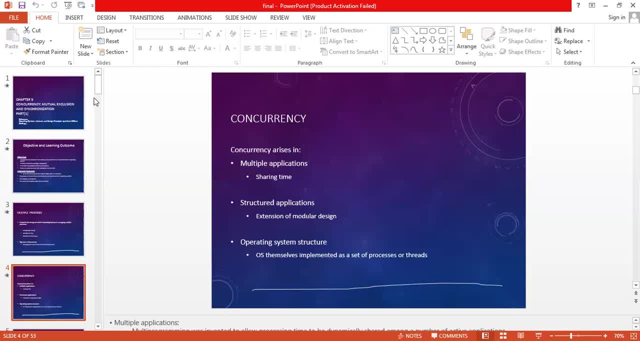 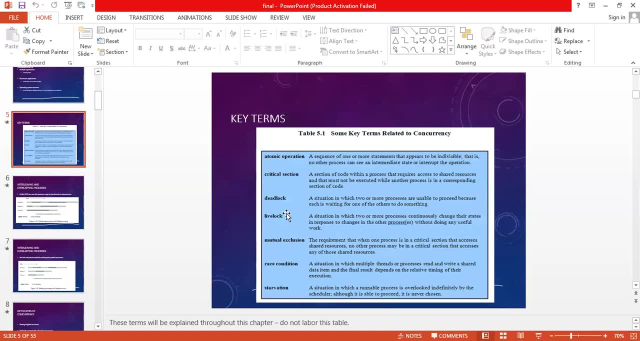 It is implementing certain set of processes or threads. Let's talk about key terms. Atomic operation is a sequence of one or more statements that appear to be individual. That is, no other process can see an intermediate state or interrupt the operation. Atomic operation is when our sequence or process is in an intermediate state of some other process. 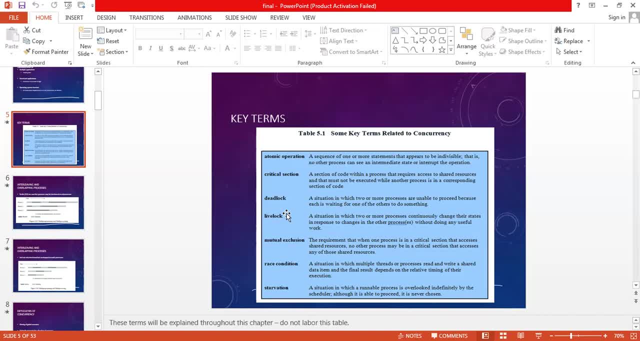 Or can interrupt it. It is not possible. In critical section there is a section of code within a process that requires access to shared resources And that must not be executed while another process is in a corresponding section of code. Critical section is a section where shared resources are required. 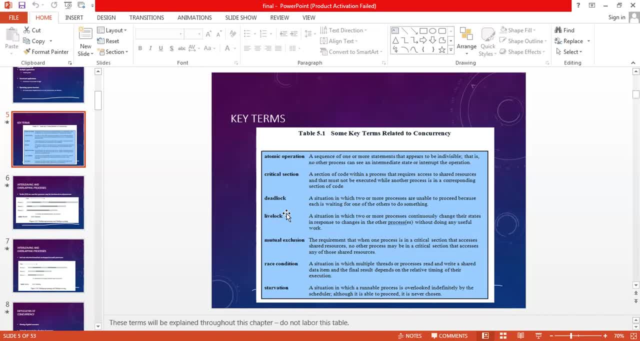 Processes are using the resources according to their needs. But at the same time, if one process is present in that critical section And there shared resources are required, Then no other process can go to that particular section. Deadlock is a situation in which two or more processes are unable to proceed. 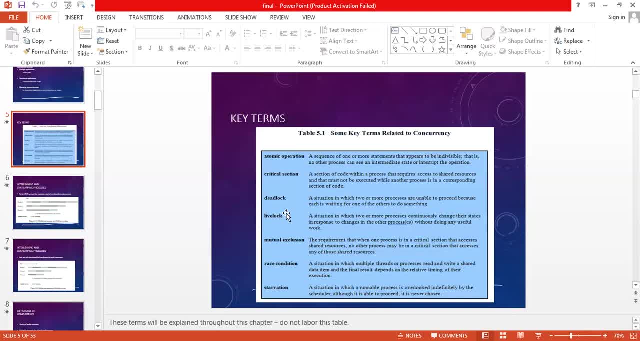 Because it is waiting for one of the other to do something. In deadlock. one process is waiting for another process to release resources, So I will move forward. P1 has resource R1 and P2 has resource R2.. But P1 needs R2 resource to run. 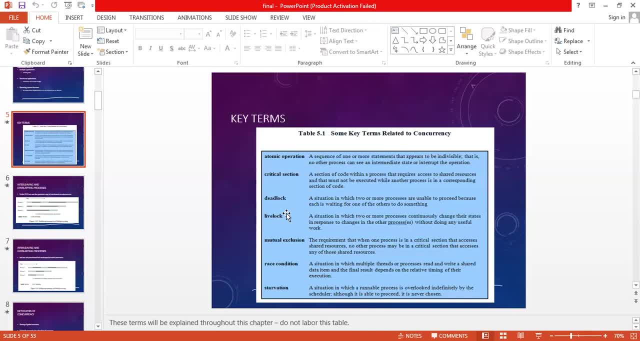 And P2 needs R1 resource to run, So both will be in the same waiting. When will P1 be released? When will P1 be released? When will P2 be released? So there will be no useful work in this way. 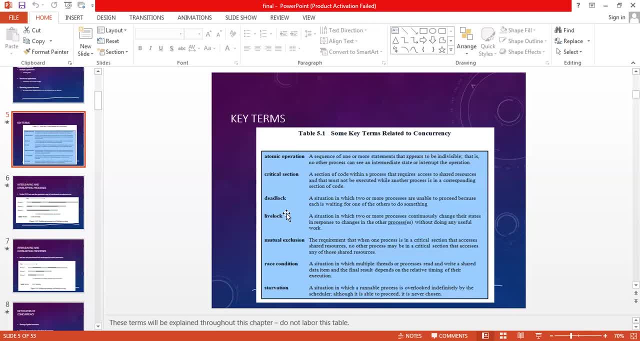 There will be deadlock. In fact, there will be no work in deadlock. What happens in live lock? Live lock is similar to deadlock. Basically, what is happening here is that the process is that our work is performing continuously. It is changing its state. 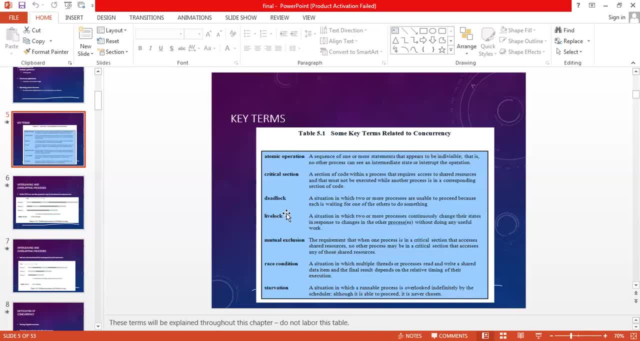 But no useful work is performing. The state changes because the process is affected by the other process and changes its state. Let's talk about mutual exclusion, The requirement that when one process is in critical section that exceeds your resources, no other process may be in a critical section that exceeds any of those shared resources. 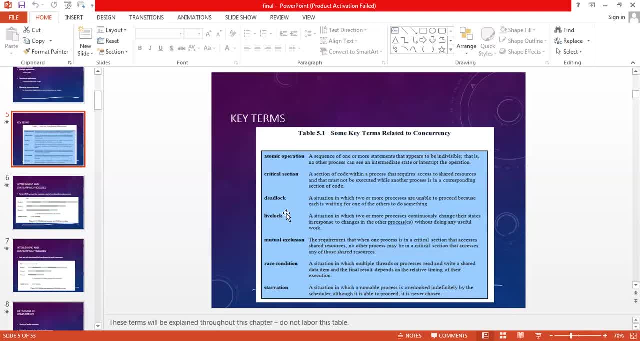 In mutual exclusion. it happens that if the access of our shared resources is provided through critical section, if any particular process is accessing those resources, then at the same time no other process can access those resources. This is the requirement of mutual exclusion. 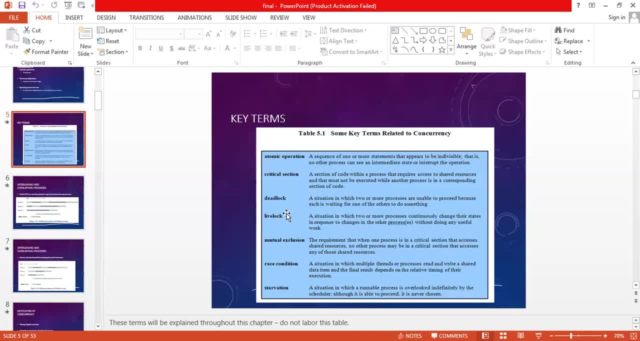 In race condition, multiple threads are processing the read and write shared data items. So the final result in race condition depends on the execution: Which process came first and who executed it. our result will depend on that. Let's talk about starvation. In starvation, what happens is that in starvation, 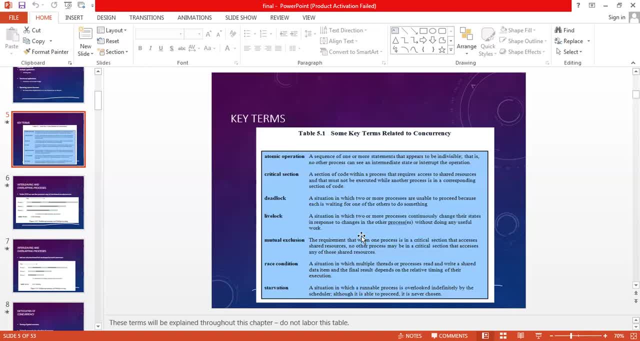 what happens is that in starvation, the priority wise, the execution is going on. The one whose high priority is executed, we execute it first, And those whose low priority is executed. the process is on waiting. In this way, what happens is that starvation occurs. 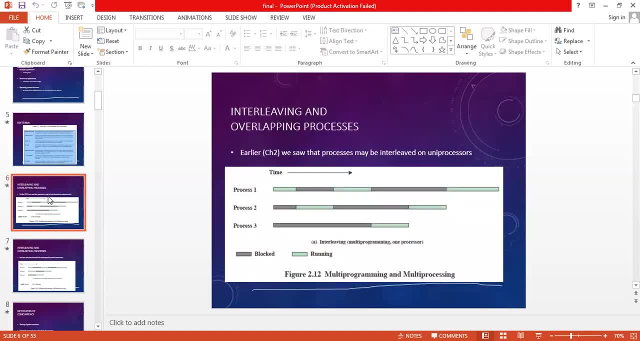 Let's talk about interliving and overlapping processing. Here we have process P1, P2, P3. And here it is being told that interliving is a uniprocessor. Interliving process is always used. Interliving process is always used. 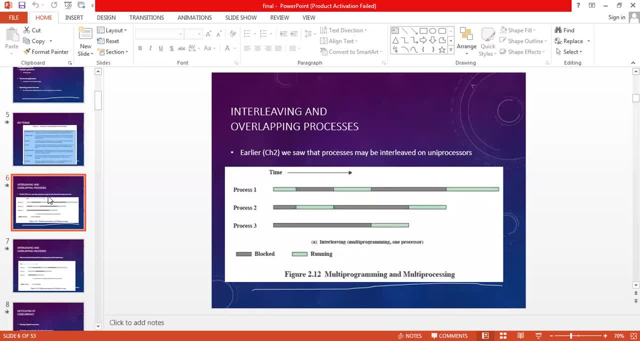 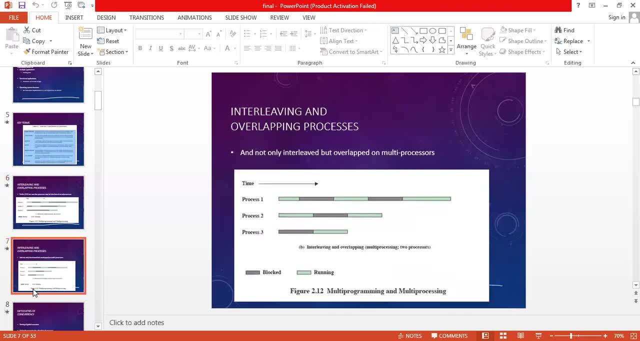 It is a uniprocessor. It is a processor in which there is only one processor. The execution is being performed there. If we talk about overlapping process, the overlapping process is working in a multiple processor. There is no one processor there. 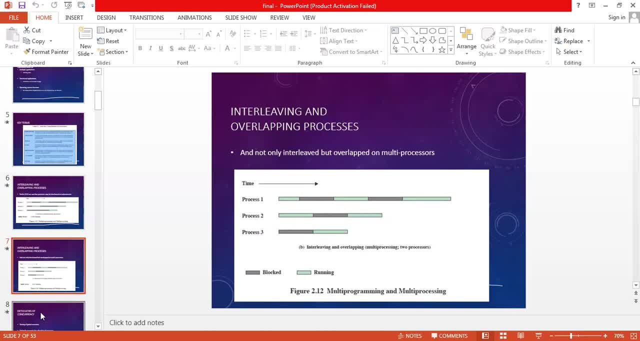 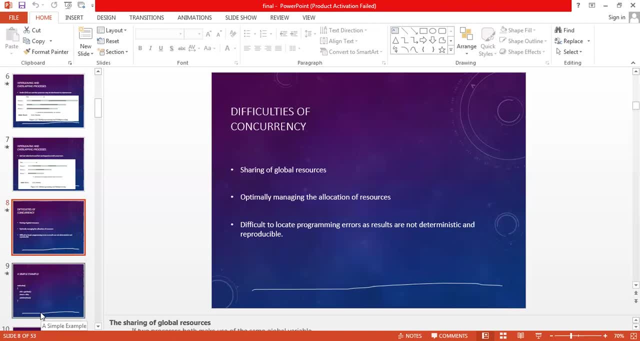 There are multiple processors there. There are multiple programs running at the same time. The difficulties that are coming are in concurrency If we talk about the share of global resources, optimally managing the allocation of resources, the difficulty to look at programming errors. 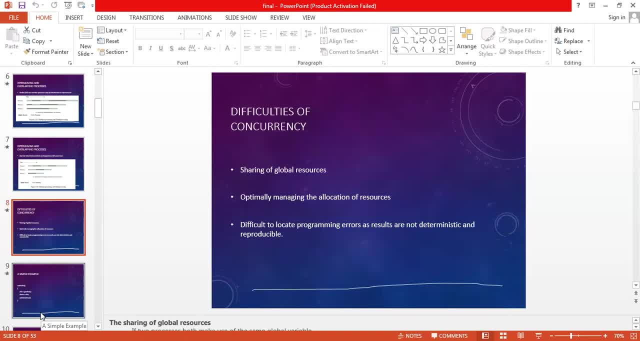 our results are not deterministic and reproducible. The difficulties of concurrency are that our resources are global. Of course we do not restrict it for any specific process. If only P1 will use R1 resources, no other process will be used. So not at all. 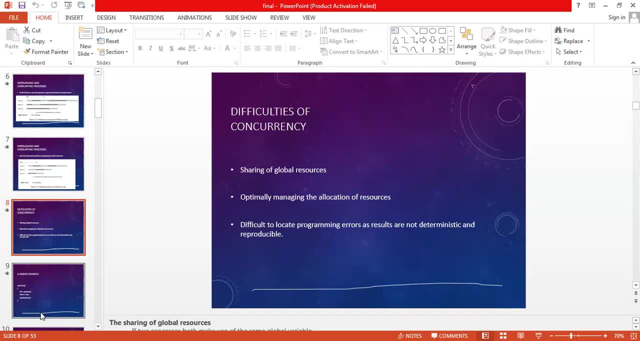 We do not do this. So if there are globally shared resources, then one difficulty comes here: Optically optimally managing the allocation of resources, that is, which resources are to be given, in which process to look at this And the difficulties that are coming in programming error. 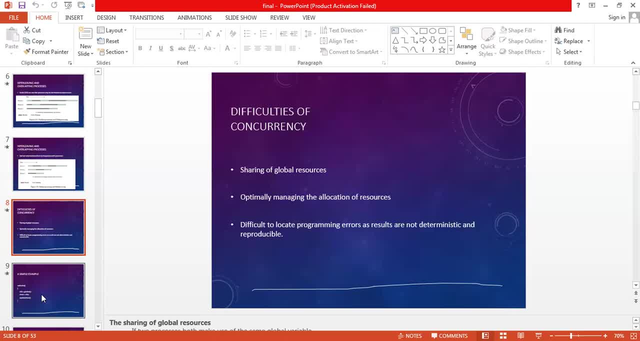 so deterministic and reproducible. that is, to determine them, to resolve them. Simple example: we have a wide echo in which we have stored the get character in and the character in is representing the character out, the character out is representing the character out. 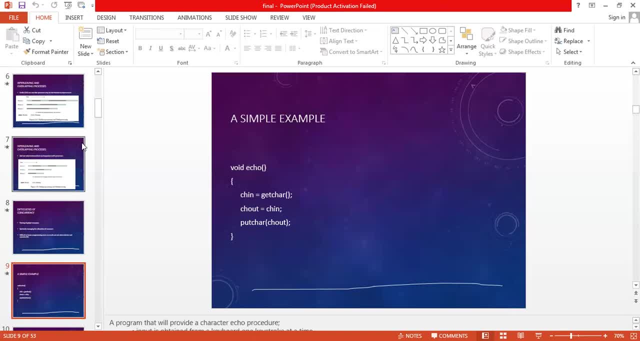 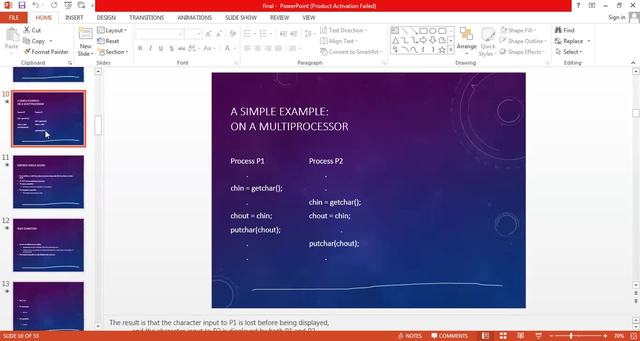 then we have taken the output from the output character. Now we have a simple example of a multiple processor. Here we have a multiple processor. it is P1 and P2.. Through the get character we have stored the character in, and the character in has been stored in the character out. 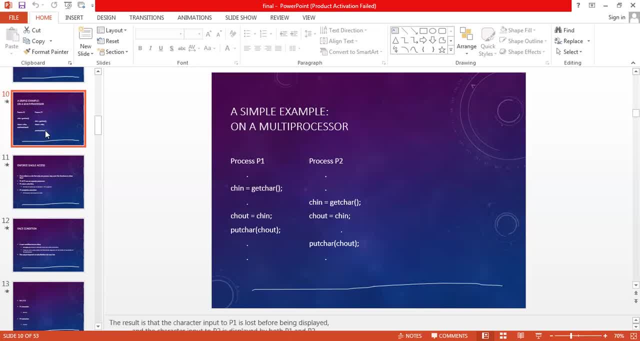 After that we will get the answer of the output character, And P2 is the same as that. Let's talk about info single access. So if we enforce a rule that only one process may enter the function at a time, then P1 and P2 run on separate process. 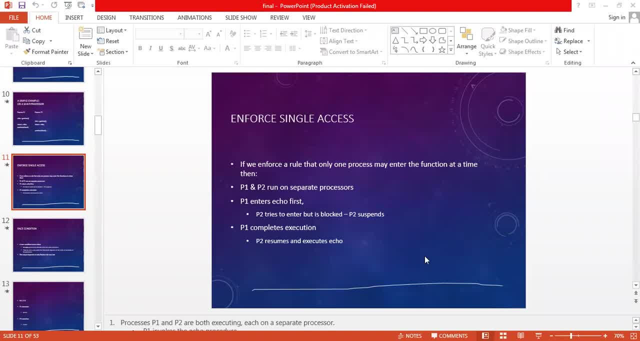 P1- enter echo first. P2- try to enter but is blocked. P2- suspended. P1- complete execution. P2- resume and execution- echo. If we talk about info single access, then at the same time we are running only one process. 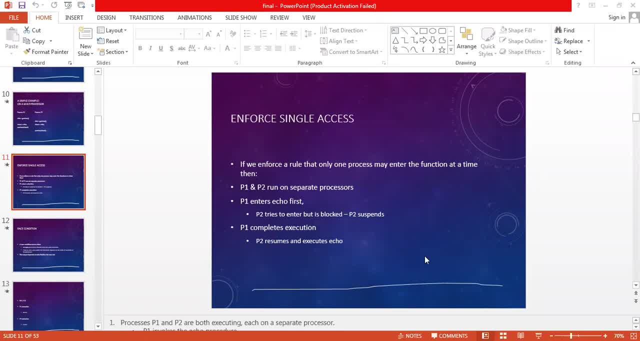 that is, if P1 process is, if P1 P2 process is, basically if we are running P1, both the processes will be running in a separate process. If P1 enters first, then P2 will try to enter the force. 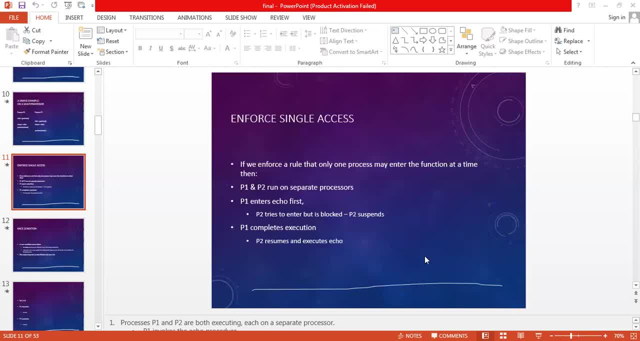 But P2 will not be able to enter because we will block it or put it in a suspending state. Until P1 is completed, P2 will not be resumed. As soon as P1 is completed, we will resume P2 and echo it. 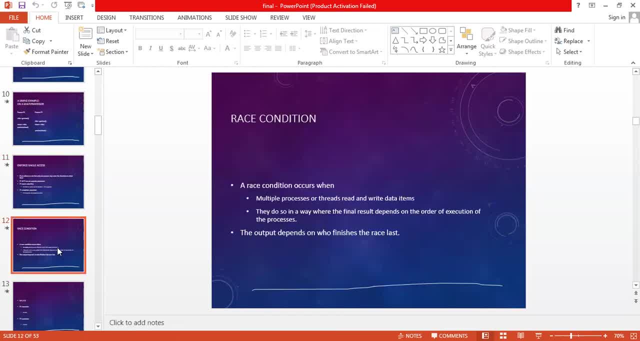 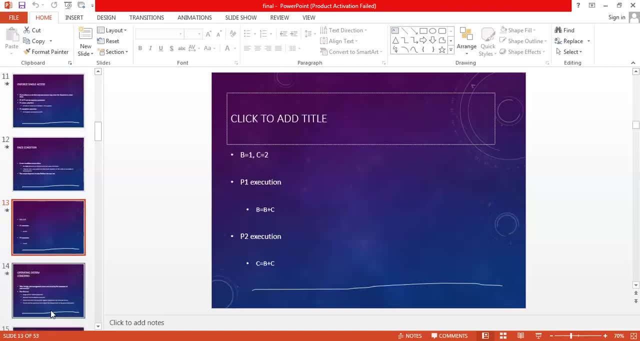 Race condition, as I told you earlier, will depend on the execution of the race condition. The final result, the process that will come first, will also be executed first, As we talk about B1,. B1 equals to 1, C equals to 2,. 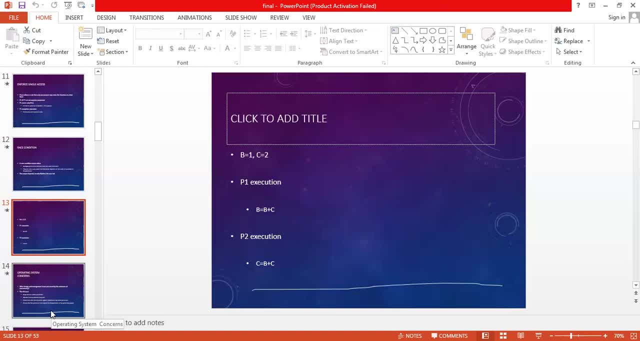 so P1 execute, B equals to B plus C will happen. If P2 is executed, then C equals to B plus C will happen. Let's talk about operating system concern. what design and management issues arise by the existence of concurrency? The OS must. 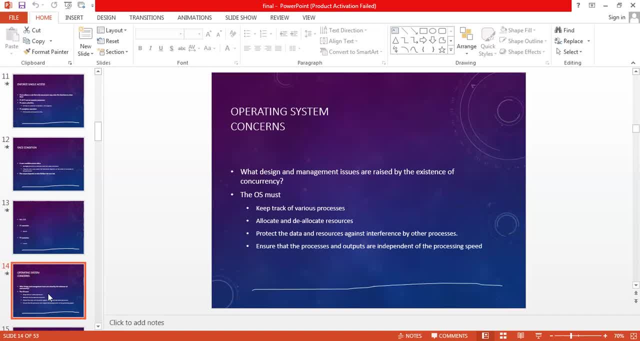 first of all, the OS is keeping track, looking at various processes, allocating deallocation. allocation means providing space in memory. deallocation means when the work of those resources or that particular process is over, it is deallocated. It is protecting the data. 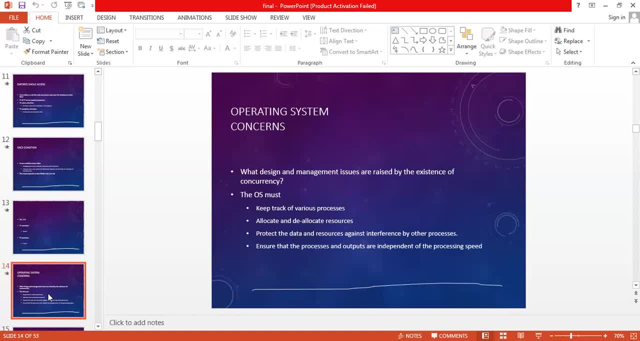 the resources. again, interface by other process means with the interaction of other process or with interference. it is protecting, ensuring that the process, the outputs, the outputs that are coming are independent. the process of speech is independent After this. 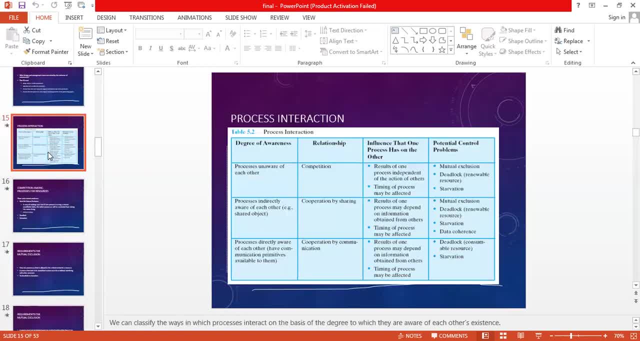 we come, we have process interaction. process interaction means degree of awareness, relationship, influence that one process has on the other, potential control problem. Here we have four columns in which we have added further information process, unaware of each other. 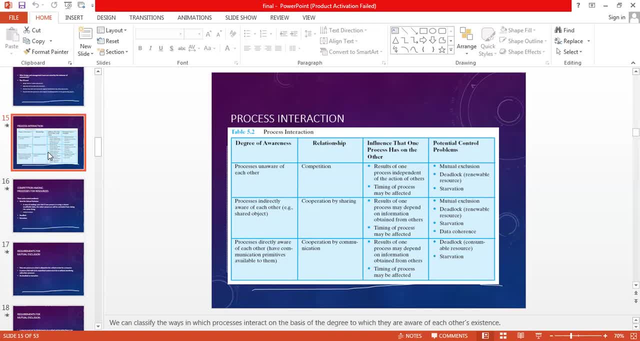 process which are unaware, in which, as I told you earlier, their relationship is competition. that is, if P1 is P2, then there will be competition that P1 will say: I will go first from P2, P2 will say: 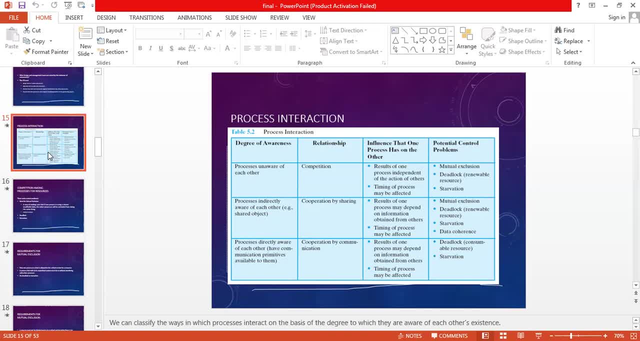 I will go first from P1, and so on. Result of one process. interaction of one process. independent of the action of other. independent of the action of other, the timing of the process may be affected. the time of the process can affect. 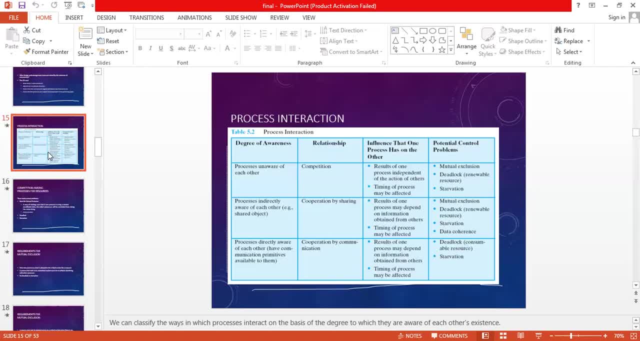 who reached first, who reached later. mutual exclusion comes deadlock. comes reservation, which I have deadlock. renewable resources. comes starvation, which I have told you earlier. process is indirectly unaware. I have told you, cooperation is happening, process is directly. 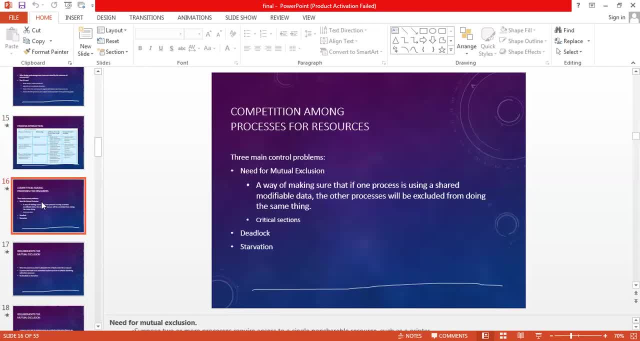 unaware, then all the results will be followed here. If we have competition among process for resources, there are three main control problems. we have need for mutual exclusion. what are our needs for mutual exclusion, which I have told you earlier that in critical section? 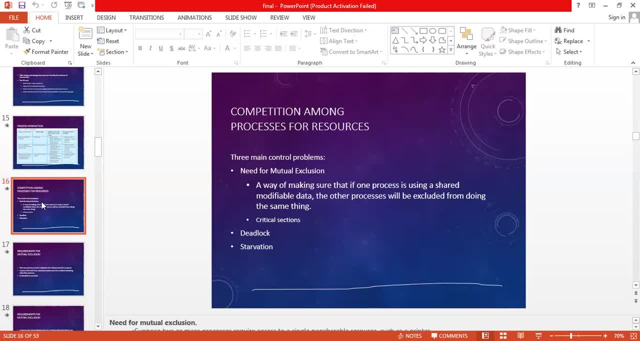 what happens is we should have only one process which is accessing the shared resources- and here also it is written- our way of making sure that if one process is using a shared modify label data, the other process will be excluded from doing the same thing. 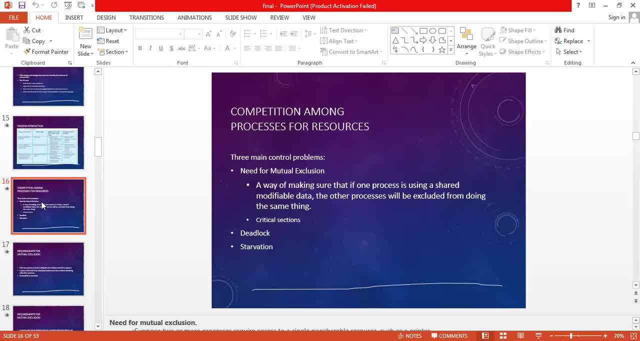 so until we exclude other process- that means to access it- we will not be able to access it. we will not be able to allow it to use the resources. and then, after that, the critical section which I have told you in the dialogue. 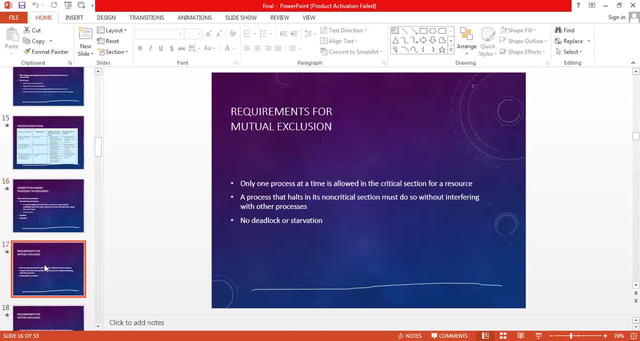 which I have discussed with you, which I have also discussed with you, which I have told you above. let's talk about requirement for mutual exclusion. as same as that, only one process at a time is allocated in the critical section for our resources. 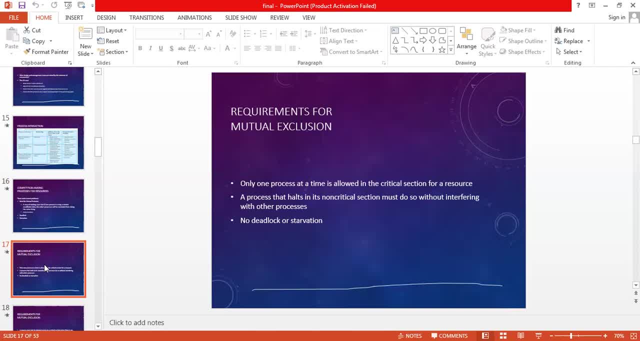 as I am repeating again in the critical section. at the same time, there will be only one process. a process that held in non-critical section must do so without interfering with other. one process will not interfere with any other process and no deadlock. 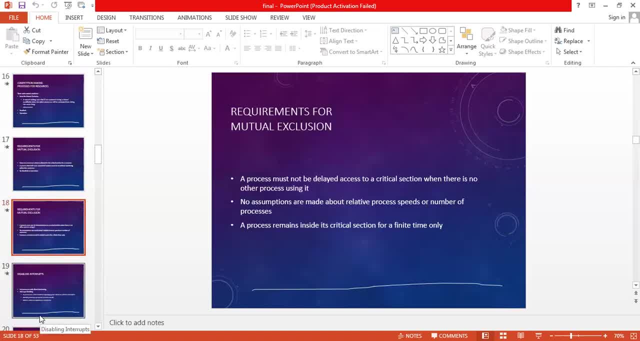 and no starvation. there will be no deadlock or starvation. a process must not be delay access to a critical section when there is no other process using it. if there is no process in our critical section, then I will not delay any process. I will not make. 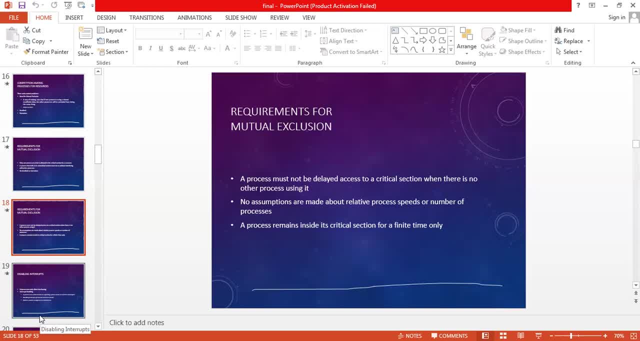 anyone wait and immediately take it in the critical section so that the process can be taken in the critical section. no assumptions are made about the relative process speed and number of process. I will not make any assumptions related to process. the process remains inside. 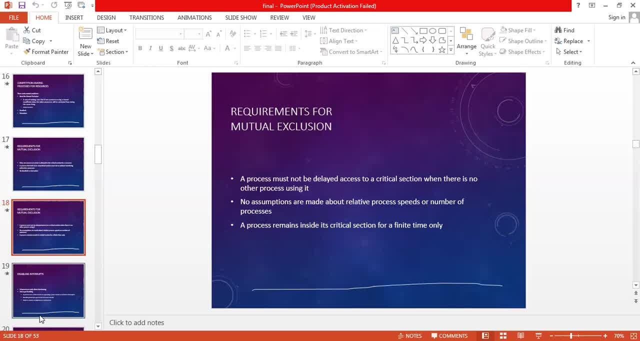 the critical section for a finite time only. the process in the critical section will be for the same time limit as it is allocated. there will be a particular time, a finite time. there will be any process in the critical section for the same time. 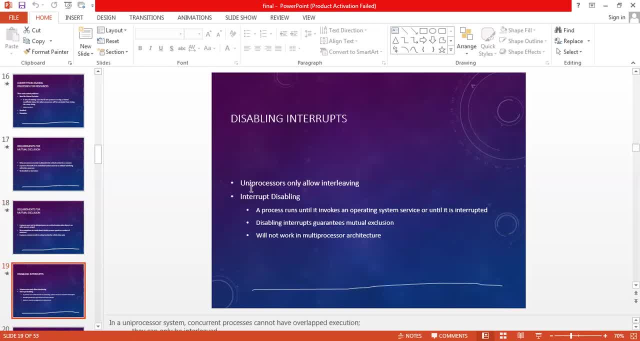 let's talk about disabling interrupt. in disabling interrupt, uniprocessor only allow interleaving interrupt, disabling a process run until it invokes an operating system service or until it is interrupted. disabling interrupt in guarantee mutual exclusion will not work in multiple process architecture. disabling interrupt: 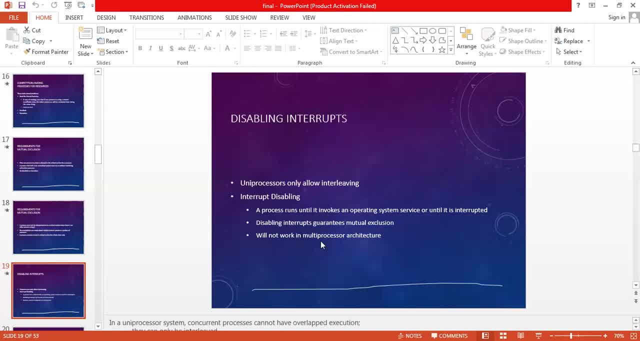 in uniprocessor. I told you. there is one processor which runs multiple programs interleaving, which I discussed with you. what is interleaving? it is only allowing on uniprocessor. so in this disabling interrupt which is invoked through operating system, 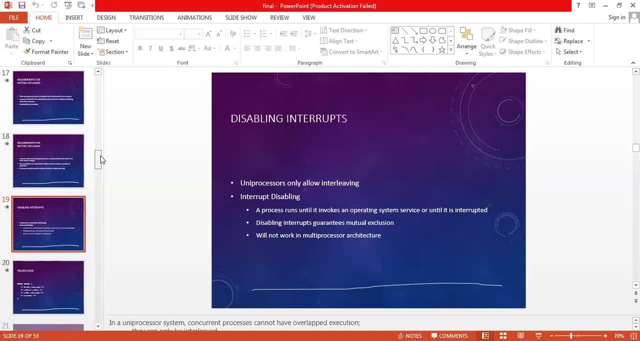 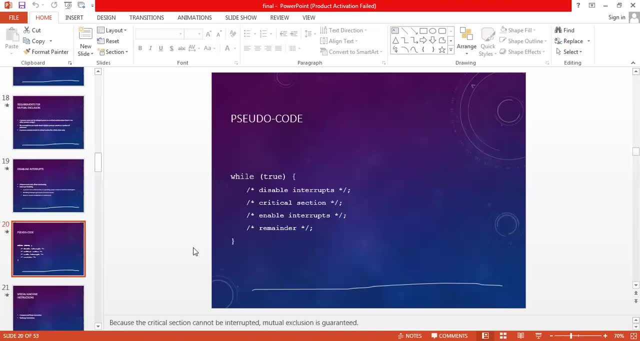 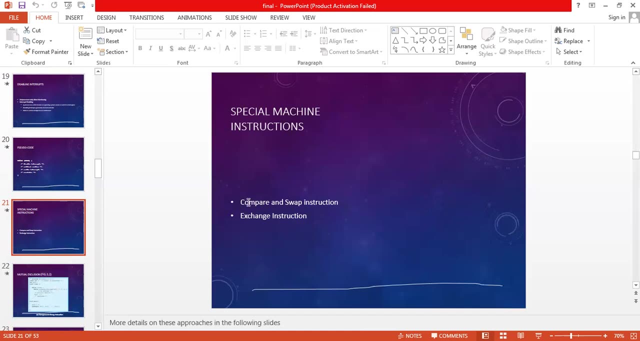 service. we are interrupting it. the interleaving will be disabled in guarantee mutual exclusion procedure. code here is disabling interrupt critical section. enable interleaving remain. it will be running until it is proved. let's talk about special machine instruction, compare and swap. 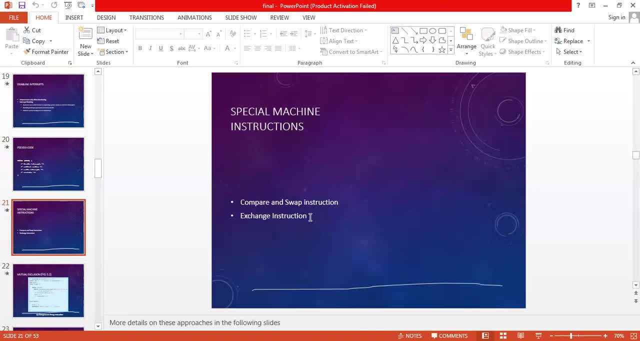 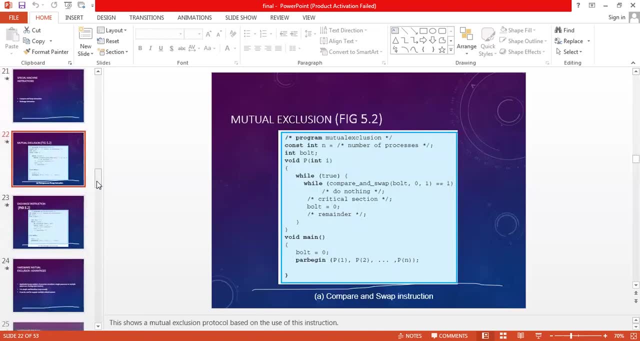 instruction: exchange instruction. compare swap instruction. change P1 to P2, mutual exclusion to 2603. If we read the code of mutual exclusion Here in front of mutual exclusion gonna, while You start from, Ed pretends while true, true involves siellä. 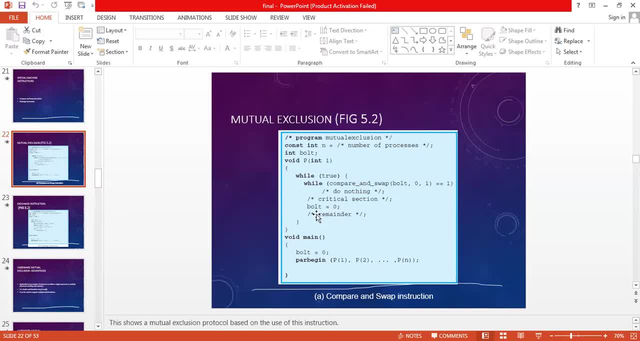 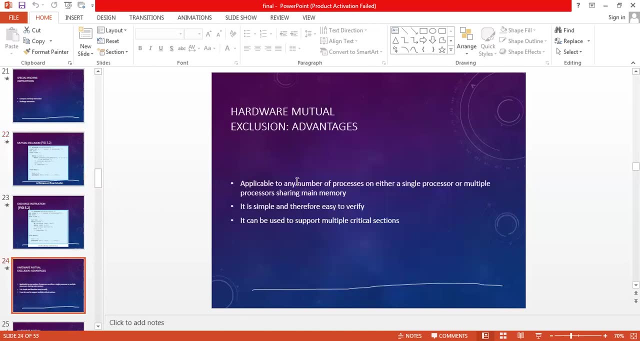 201 Circle One degrees Move. the section is going back and forth is a livable on P1, P2, P3 Probe, Playing after that to any number of process or either single process or multiple process sharing main memory. it is simply and force easy to verify. it can be used to support multiple critical section. and this is one of the advantages of hardware mutual- is that we are supporting multiple critical section, means we are supporting multiple critical section and it is simple and easy to verify and we are sharing main memory. and other than this, the disadvantages of hardware mutual is that it is busy waiting with consumer and the time of consumer process is very long and it is busy. 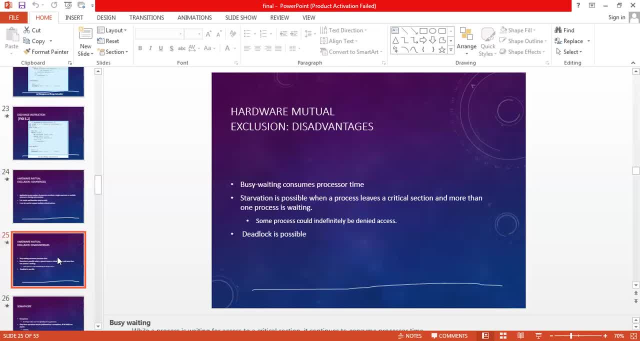 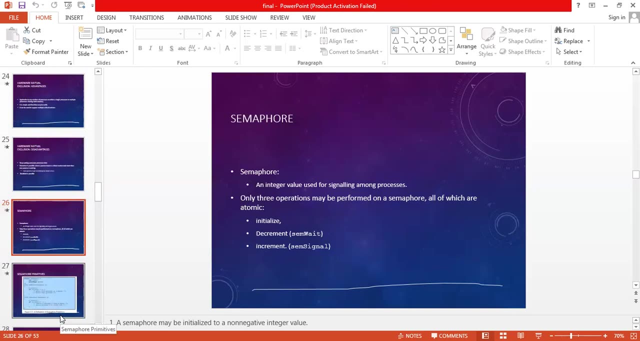 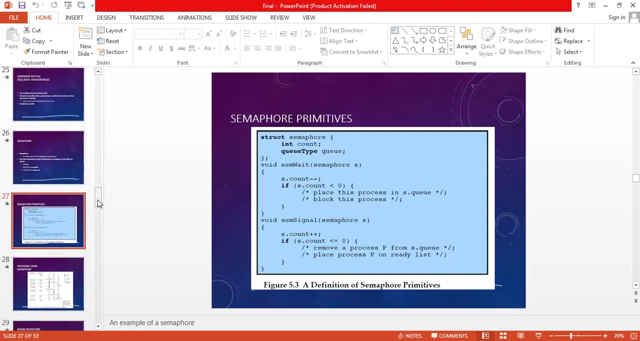 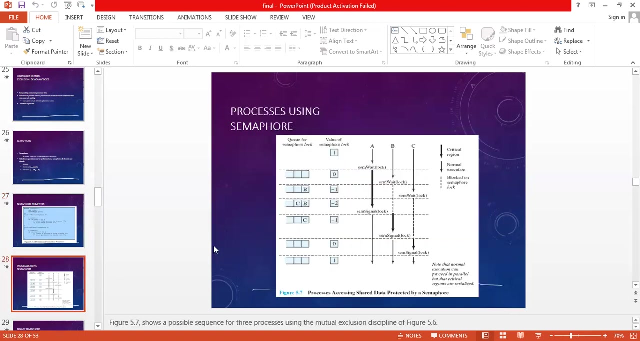 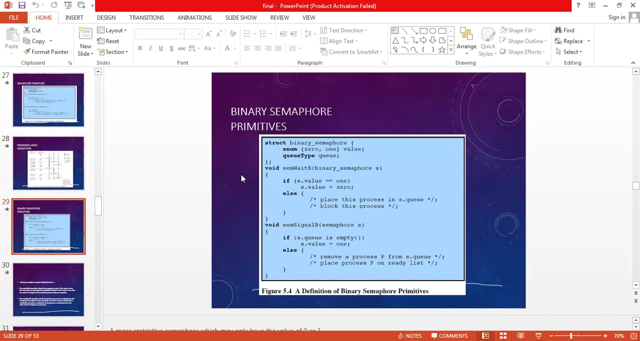 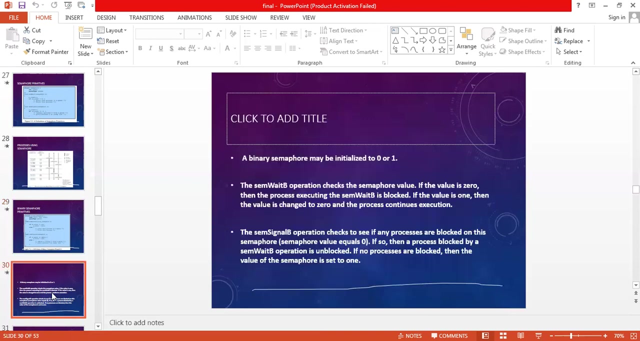 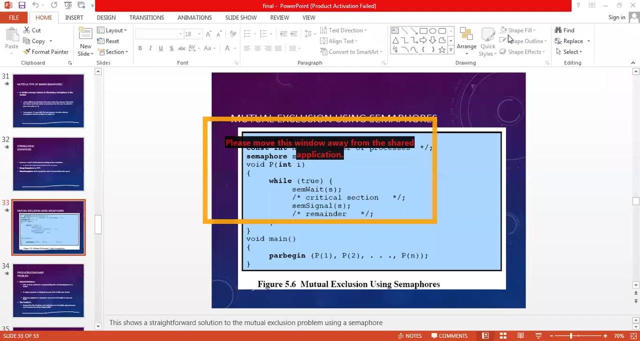 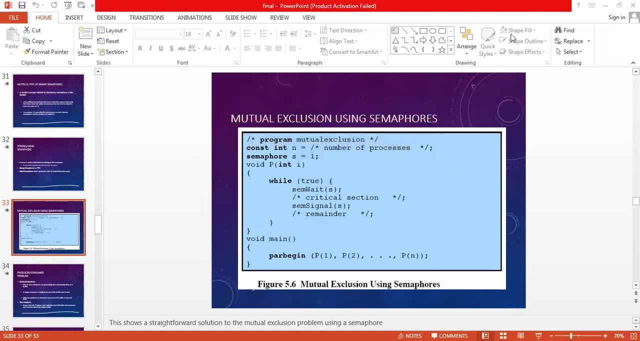 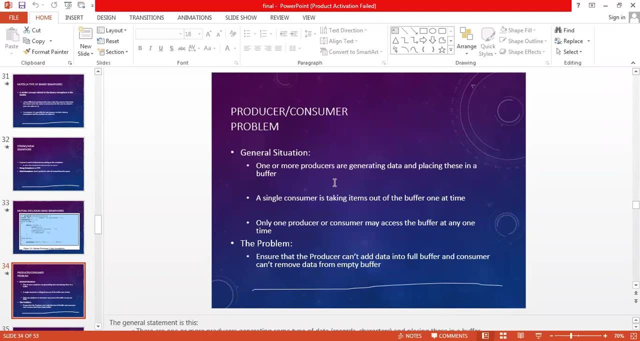 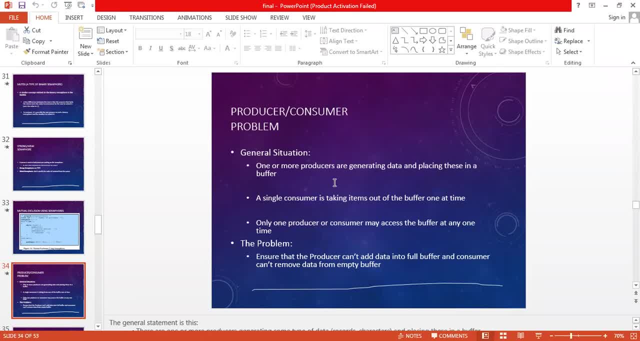 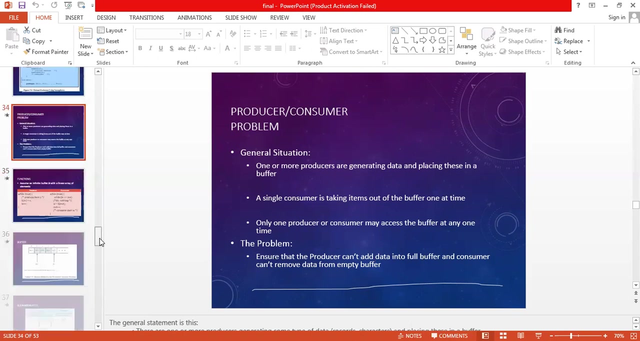 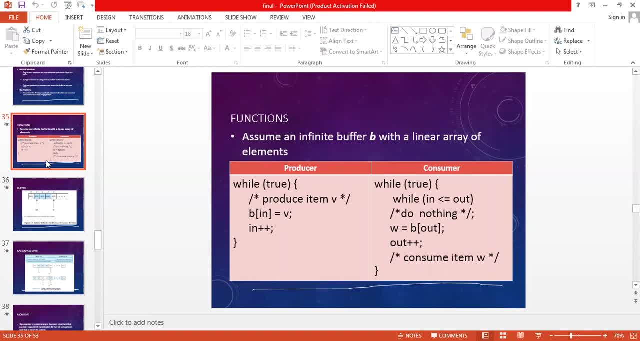 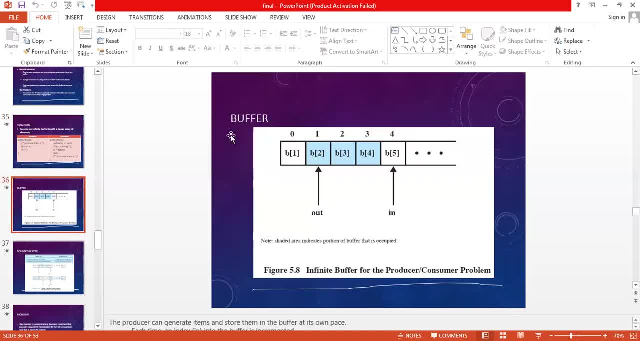 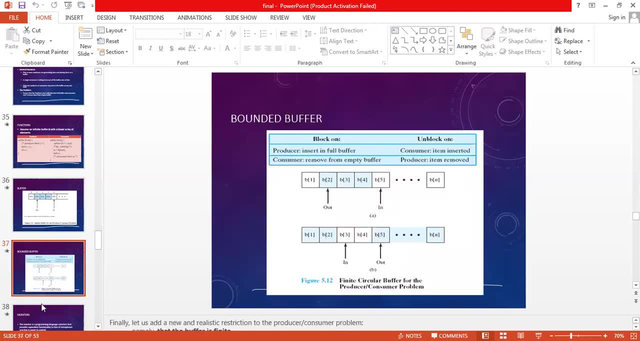 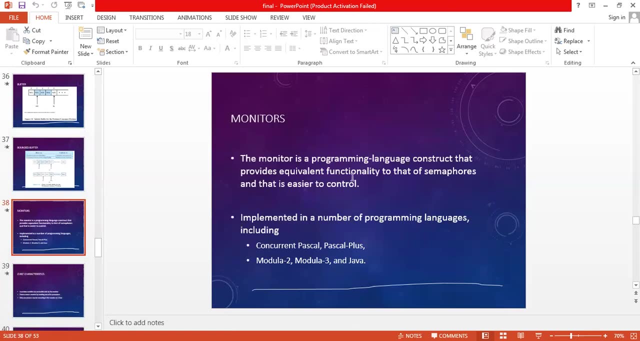 same as that. here we have a diagram which is getting diagrammatically out and this is getting in from here. this will get out from here, same as that of bounded buffer. this is the explanation. let's talk about monitor. monitor is a programming language which constructs provides equivalent functionality. 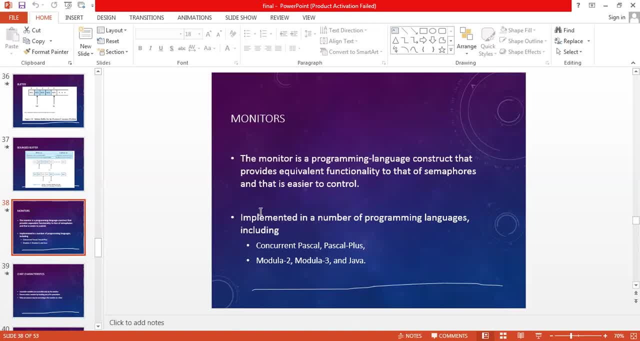 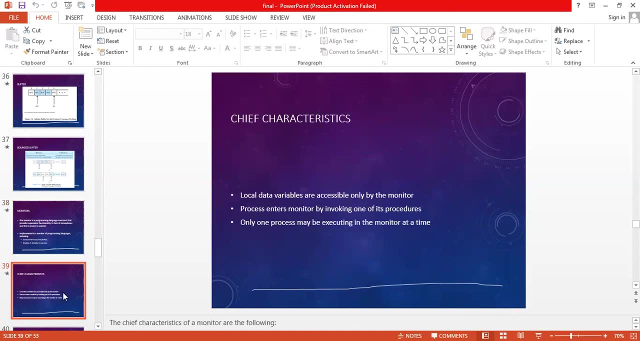 with the help of semaphores and their basis to control. to control implement number of programming language in which concurrent is Pascal, Pascal plus Modula 2, Modula 3 and Java. after this we come to the chief characteristics. local data variables are accessible only by the. 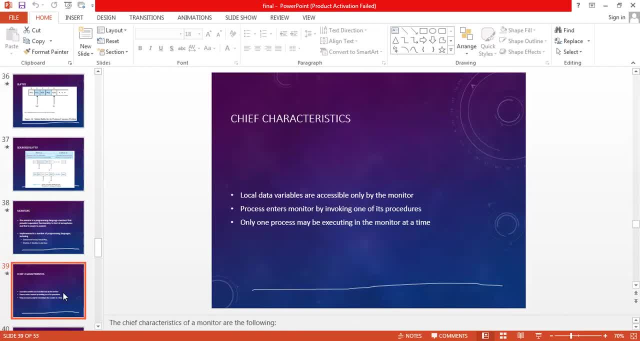 monitor process- inter monitor, by invoking one of its procedures and only one process may be executing in the monitor at a time. at a time, in the monitor, only one process will be executing process which are entering in the monitor invoking procedures, local data variables which are accessible by the monitors. 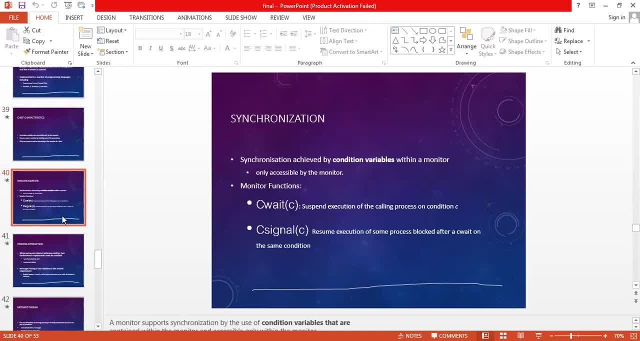 after this we will proceed further. let's talk about synchronization. synchronization is achieved by condition variable within a monitor. achieved by condition variable only accessible by the monitor. only accessible by the monitor. if we wait for C, there is a suspending execution. if we do C signal, it will resume. 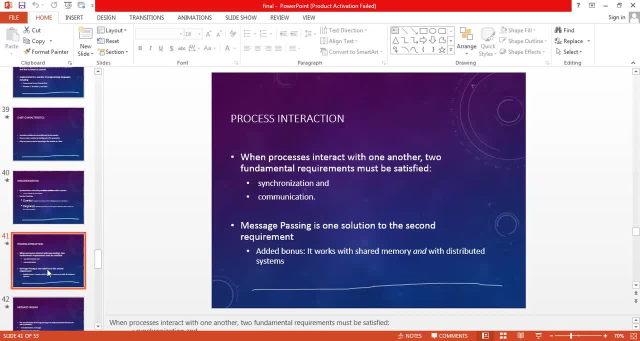 let's talk about process interaction. when one process interacts with one another, two fundamental requirements must be satisfied. when our process interacts with one another, two fundamental requirements must be satisfied: synchronization, communication synchronization. I told you earlier, message passing is one solution to be. second requirement: through message we are passing. 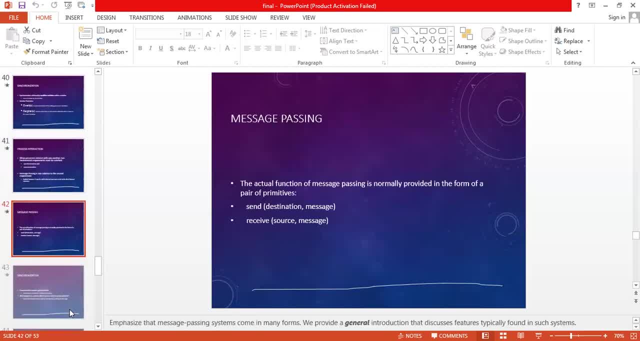 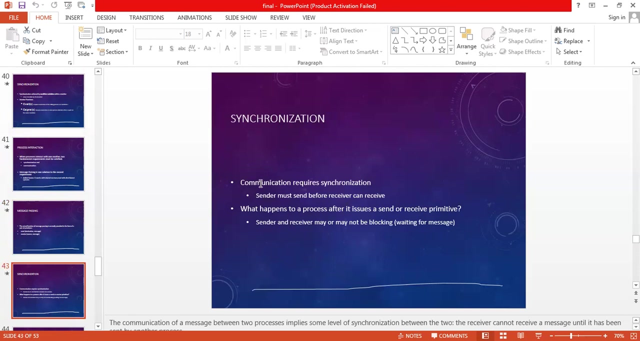 requirements and solutions we are getting ad bonus. what is message passing? message passing is an actual function to pass a message, normally to provide form of peer or primitives. we will send from destination to message, from source to message. synchronization communication- communication requires synchronization. communication requires: sender must send. 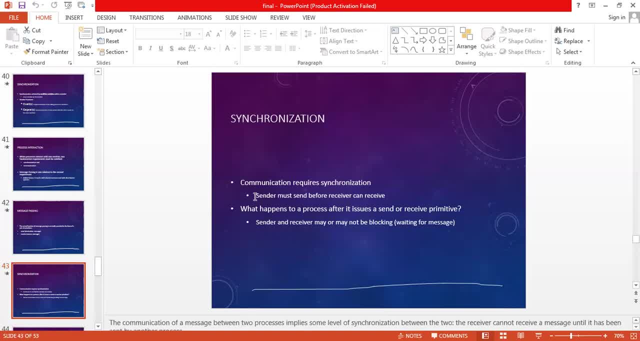 before receiving: sender must send before receiving. what happens to process after issue: sender receive. primitive sender and receiver may or may not be blocking sender and receiver ho bhi sakta hai, nahi bhi ho sakta hai, waiting for a message ke liye bhi kar sakta hai ho. 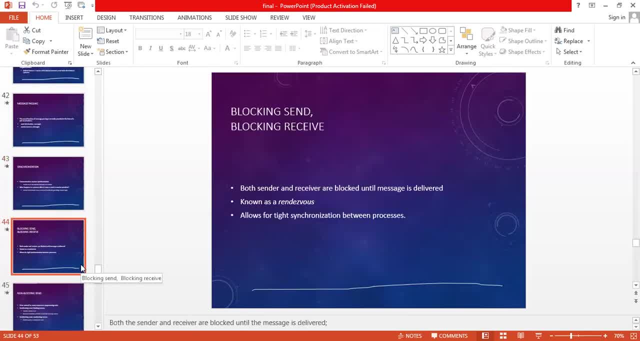 sakta hai chike block and send blocking and send or blocking receive, agar both sender and receiver jo hotein block ho jai until message is delivered ke sabte ke ma message, delivered now to known as written written via isko, hum written via kenge ke ab hamara. 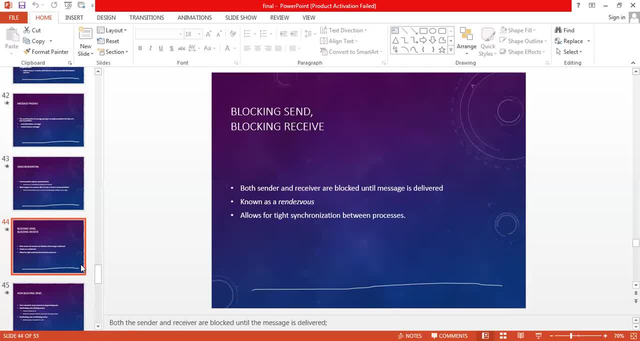 sender jo hai or receiver jo hai, wo dono hi blocked ho jai chike, until message is delivered. ke message delivery nowa ta abhi tak allow for type synchronization between process. type synchronization ho rhi hoti hai non-blocking bhi ho sakta hai non-blocking. 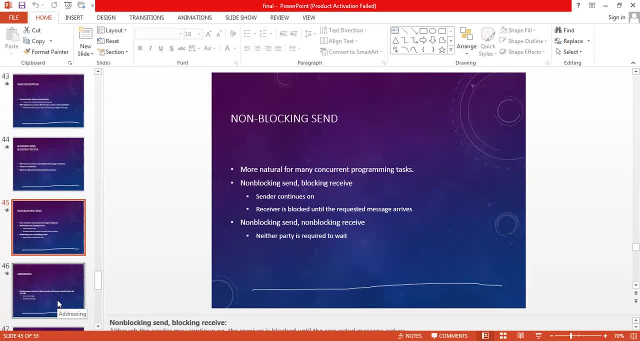 mo kya ho jai ke more natural hota hai ke concurrent programming stocks jo hai non-blocking send, blocking receive sender continue ho jai receiver jo hota hai jisne receive kia hai message wo block hai until the request message arrived. upti ke ma request message. 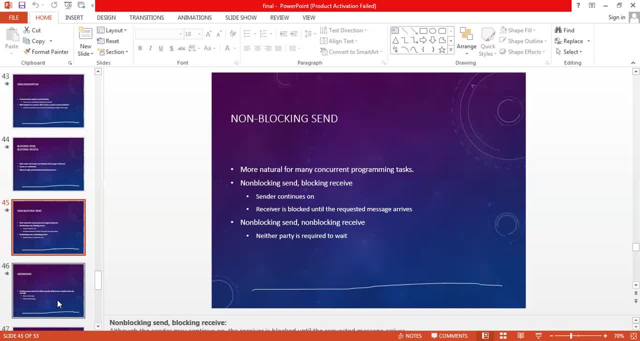 arrived nowa receiver. blocked ho jai. all are possibilities In non-blocking send. non-blocking send karna. non-blocking receive bhi ho sakta hai. neither party is required to wait. kisi bhi party ko yaani ke na sender, ko na receiver hai kisi. 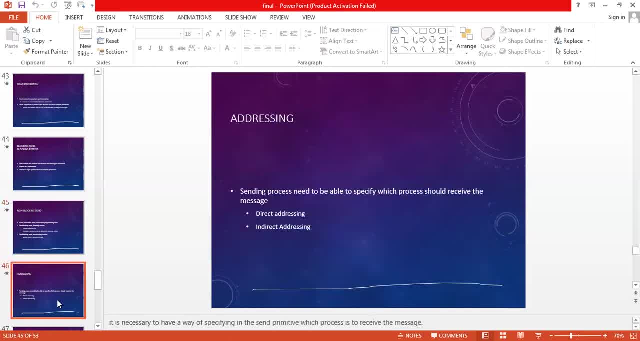 ko bhi wait na karna pahe to all are. things are depend on the situation ke humayi pa situation. kya hai? addressing ki baat karte hai to sending process. need to be able to specify which process should receive the message: direct addressing or indirect addressing: addressing as normally. 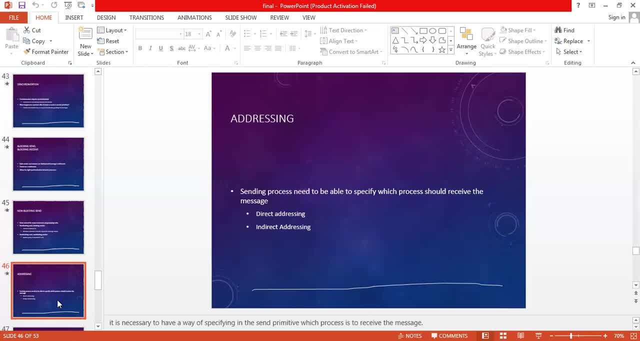 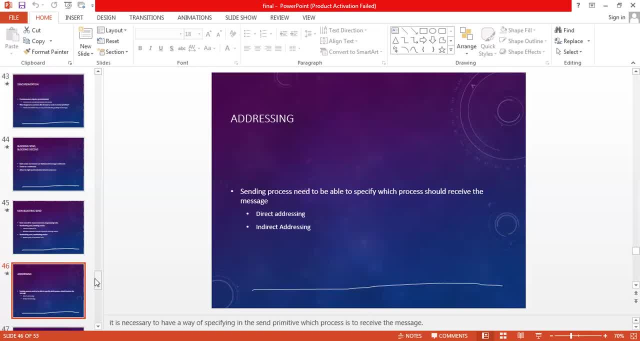 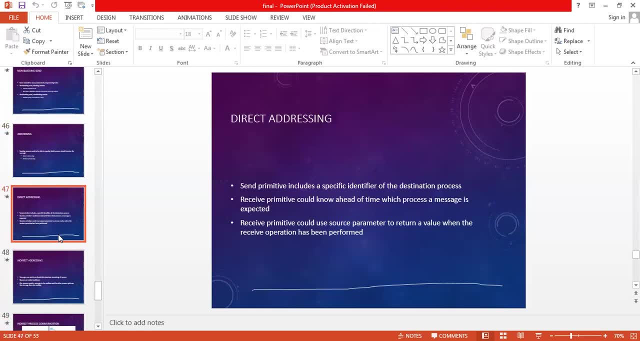 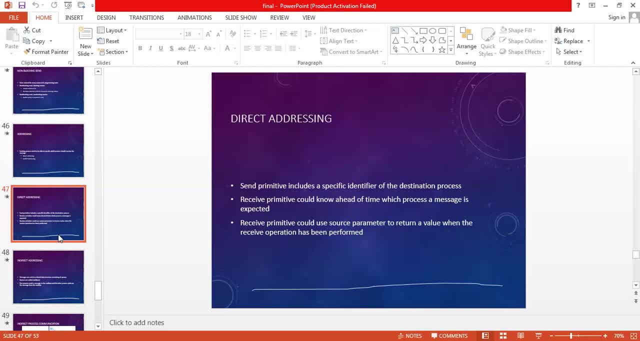 Ex codes like an indicator to send the message we send. go with a buzz mostly but whether help materials We have to know in that case as well. that is сек characterization. Just like a buzz mux goes with upland conditions job a lot. 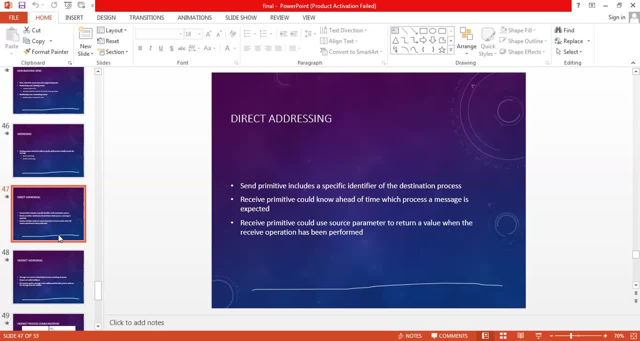 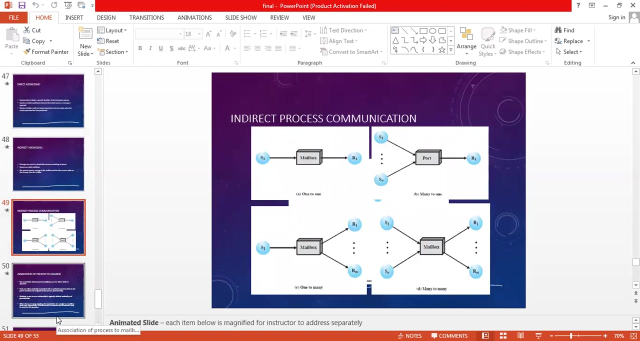 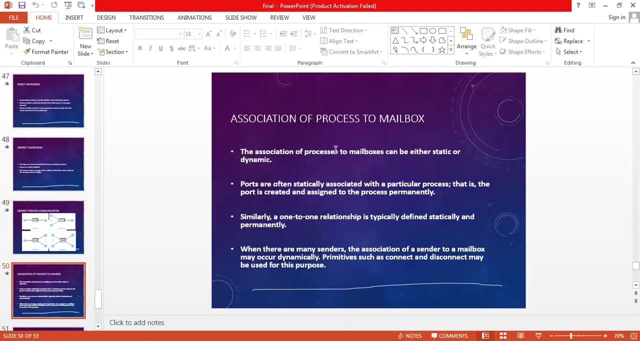 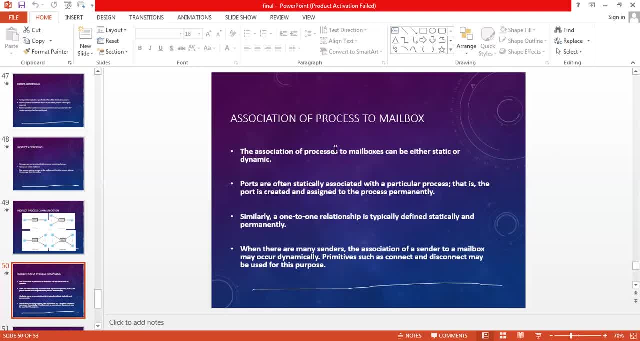 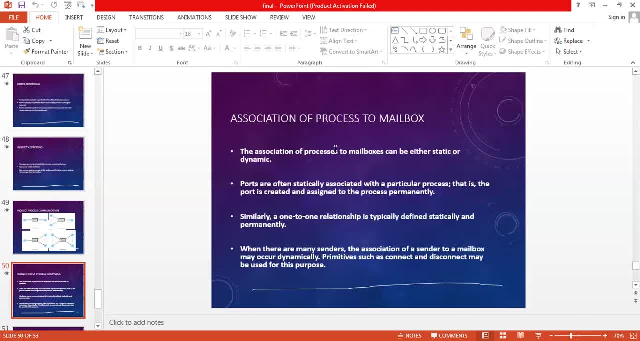 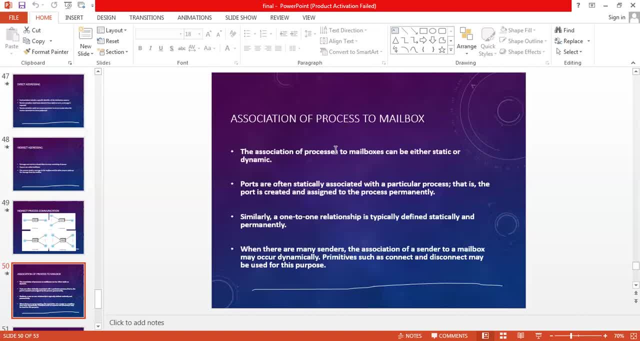 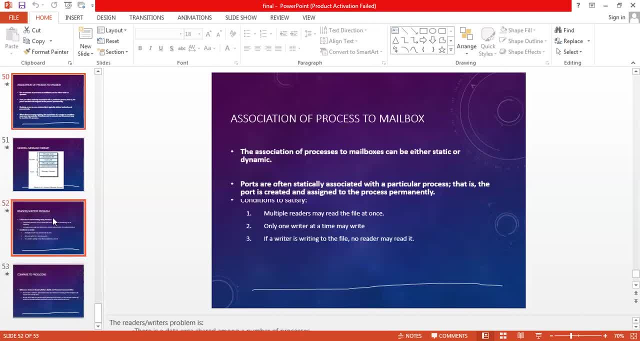 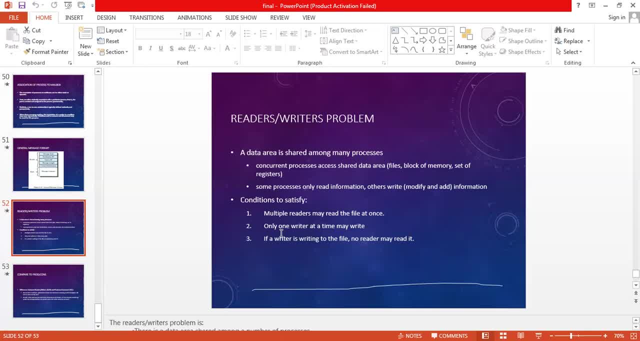 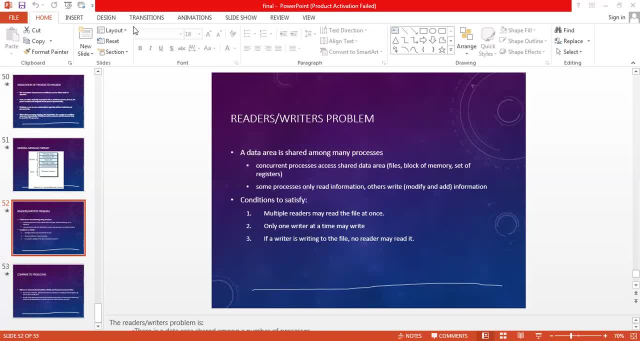 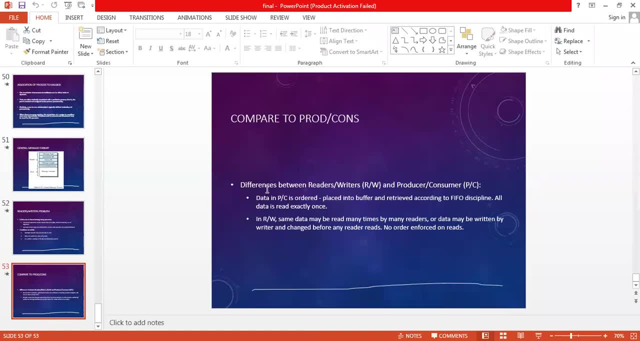 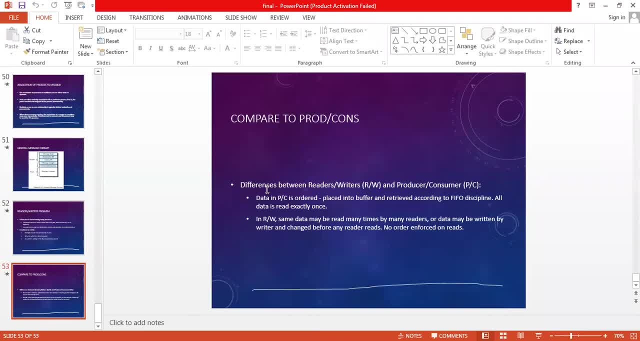 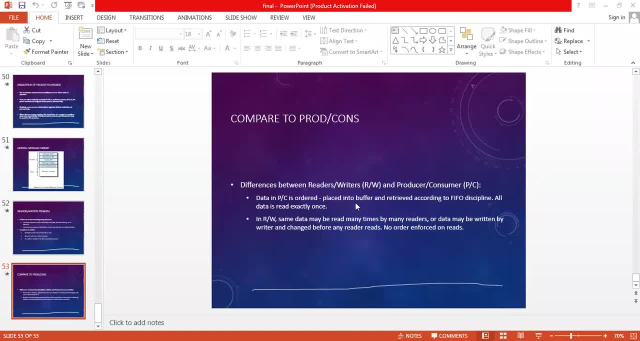 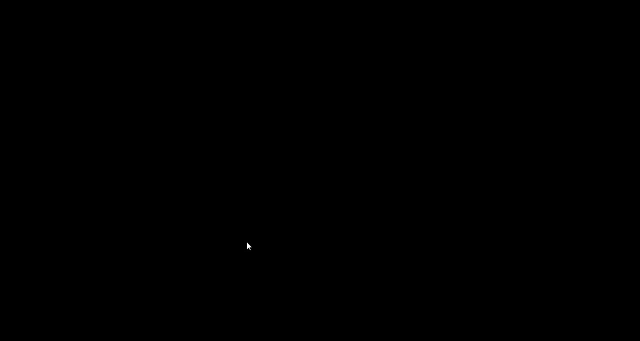 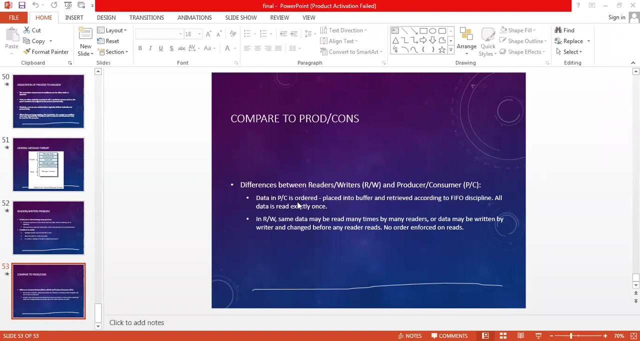